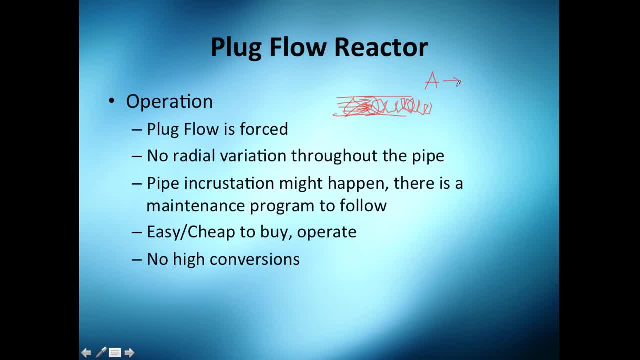 mix, and if they mix that's good, because we need A in contact with B so they can form C. that's an example. so there's no radial variation throughout the pipe. so if you will have this diameter here, you will suppose that the concentration throughout the levels even 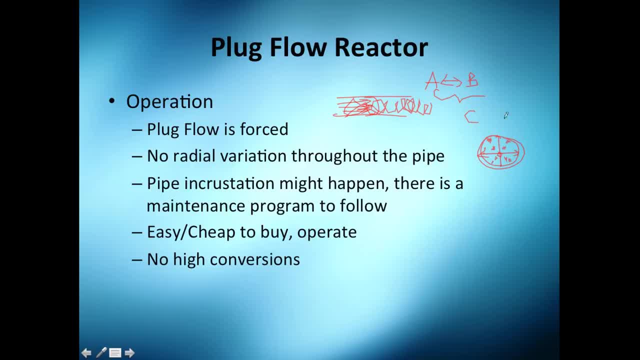 though it's near or away from the center is the same also. that's kind of ideal. but okay, we need to start with something, guys. the piping crustacean may happen, so there is a maintenance program to follow. so, yeah, you have it here and starts getting in crustaceans here and eventually it's going to. 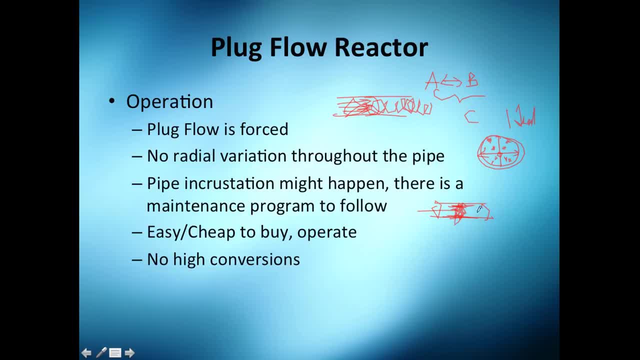 be I don't know something. very they start. you need to take it away because then your pipe is going to have corrosion or worst, your reaction is not going to be carried or, if it is carried, not with the percentage of the reaction. it's not going to be carried. it's going to be carried. 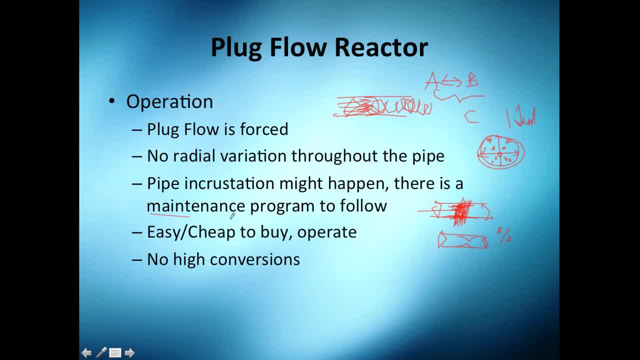 because then your pipe is going to have corrosion or worse, your reaction is not going to be carried. still, you want or conversion. so yes, you need a maintenance programs to take care of that. the good thing here is that it's easy and cheap to buy and operate. so, yeah, you got this pipe you need to. 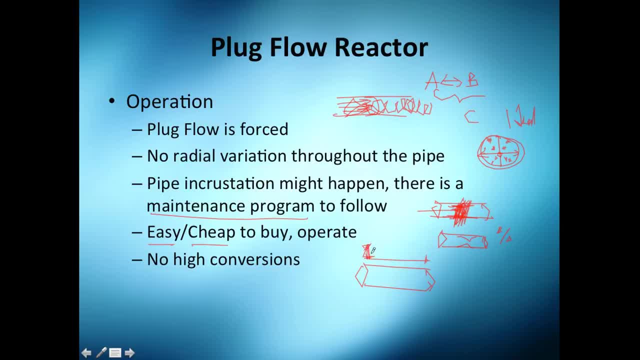 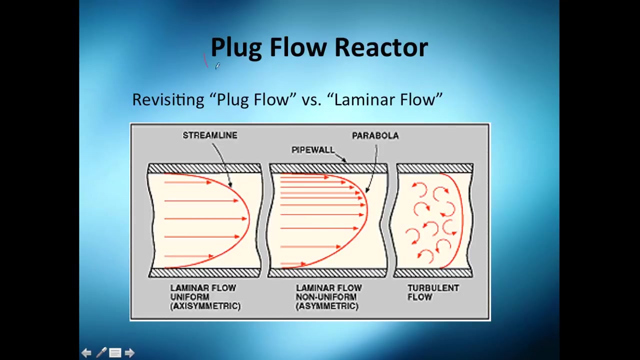 calculate the diameter, the size and how much flow do you want to get and how much product you want to get, and you just buy it and operate it. the bad thing: there are no so high conversions, such as in batch reactors, but, yes, typical in the industry to have this. so one thing I do want to remark is this: 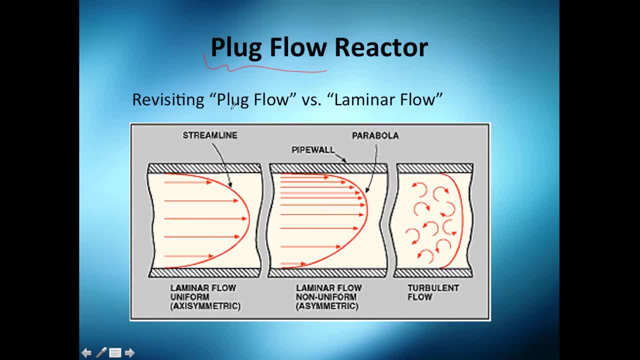 plug flow stuff. so if you've seen transport phenomena or pipe flow or mechanic fluid mechanics, you should remember that this is the typical linear velocity flow. you can see the more near the wall or the nearest to the wall or the nearest to the wall or the nearest to the wall or the nearest. 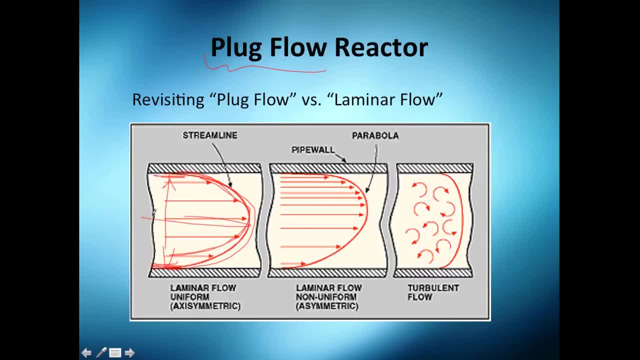 the wall is the lower velocity and in the center you got the fast. you could also heavy as a metric distribution. but what do we want here is essentially to get a plug flow like this. we want this eddies or these formations here because they are going to mix letter a or B and C. they mix them. 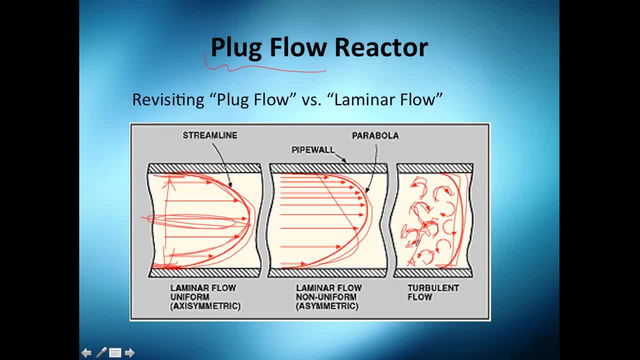 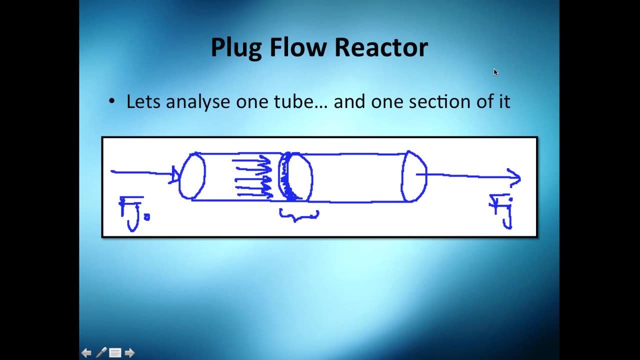 and make sure it's good for reaction. so that's why we like to have a plug flow reactor. not only that, we also want to have fast fluids. we don't want slow fluids in pipes, so that's why we're going to pump it and they mix themselves and you take them away. so that's about theory. 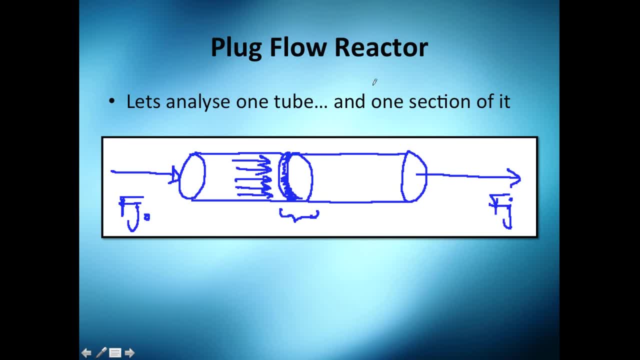 now let's do some applications of the general mass balance equation. so let's suppose we have this pipe. I'm going to cut this back and you can see there's a inlet flow here and outlet flow here, A, and here goes product B. Now, as you can see here, the velocity profile is as a plug. 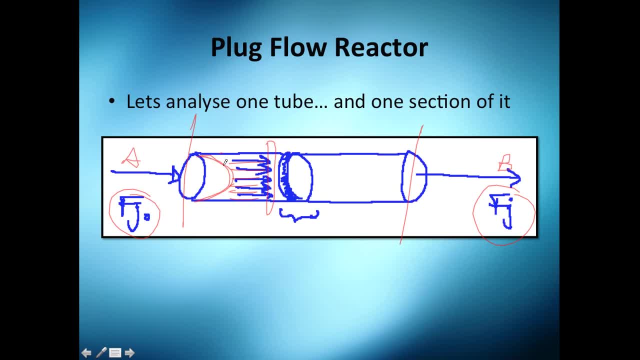 you don't have this beautiful arc which is typical for laminar. we are in turbulent case, so we have this profile. Now, if I wanted to cut this little disc- and probably you are asking why I am cutting this- the problem is that the concentration is changing with. 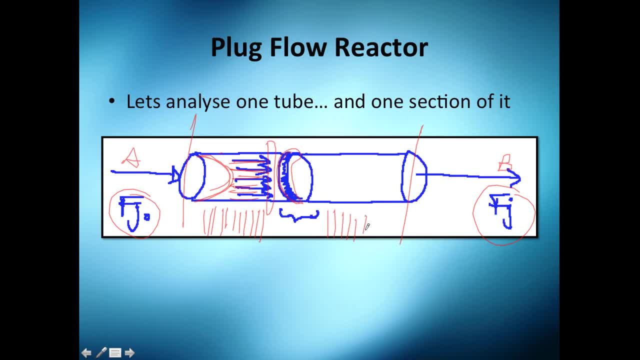 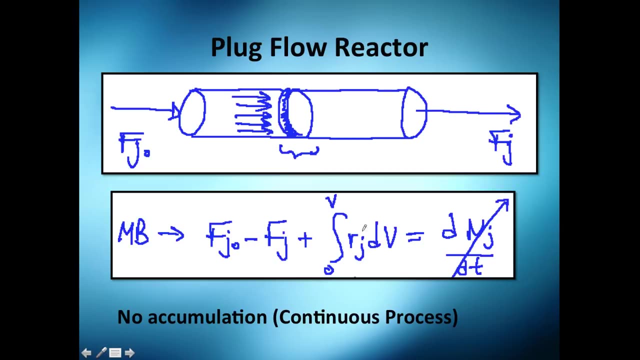 length. so I need to account for that. and one thing I've seen before in mathematics is that if you do an analysis in a small, infinitesimal part, you can apply it throughout the system. so let's do that From the mass balance. I got- yes, I got- an inlet. yes, I got an outlet. 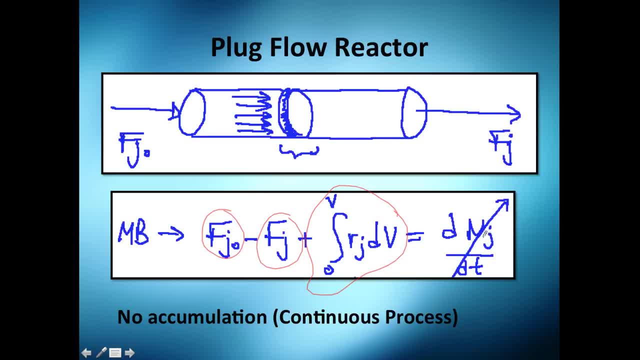 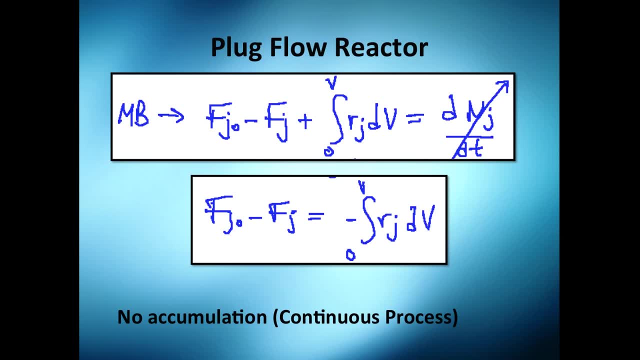 because there is a reaction- Ok, Ok. Ok, I got the generation term- and because it's steady state or a continuous process, there is no accumulation, so this is zero. So essentially, we are done with this equation. this is zero. 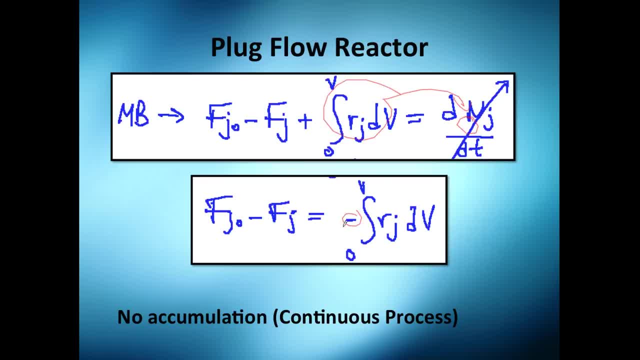 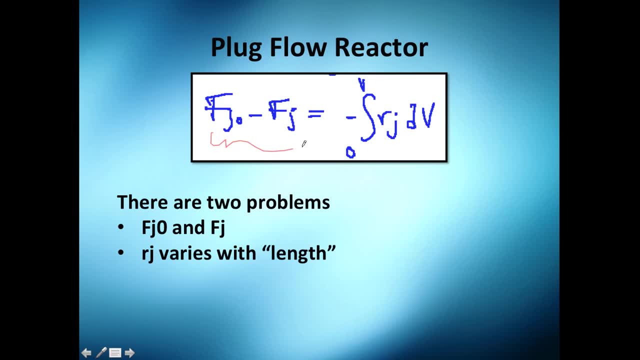 so I send this to here subtracting. so that's why the minus term. and yeah, We got this equation and we have two problems. actually, these are not that much of a problem. the real problem is this one here, because the rate of reaction does actually change. 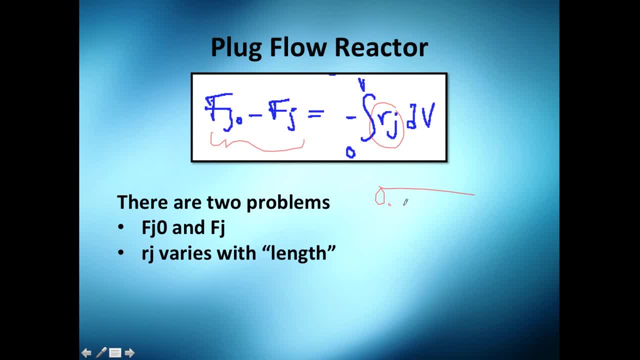 with the length of the I would say, let's say, with the reactor. so if the length changes, you know there is a length and we have a transversional area here- we're going to have volume. so, yeah, as volume changes we are changing the rate of reaction. so, for example, a typical 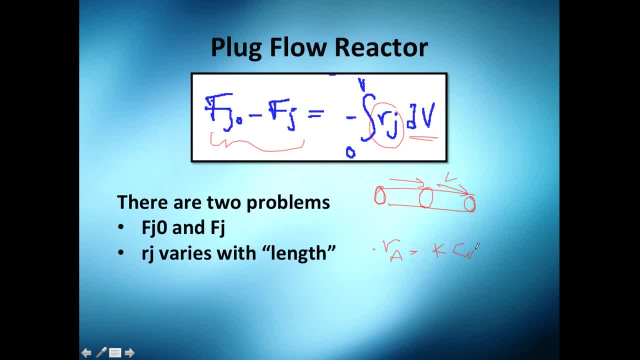 rate of reaction. law would say that k times the concentration of A. so we calculate the concentration here And the concentration here we will have different rate of reaction. so we will have kCa0, and we will have another rate of reaction here, kCa. 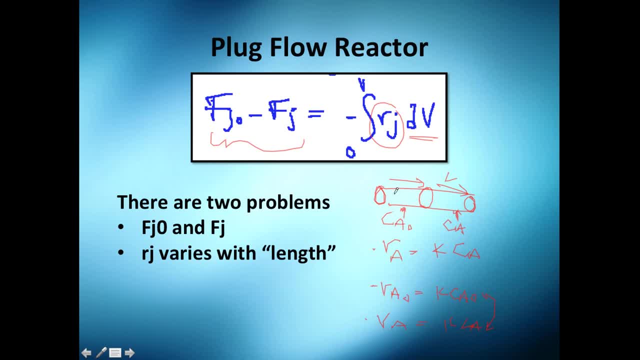 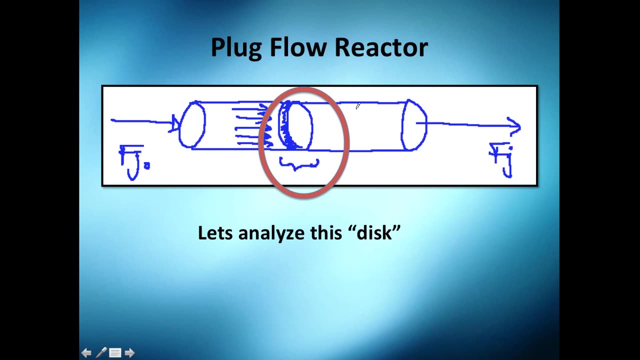 So, as you can see, the point of the reactor is, of course change the concentration with length, so the rate of reaction is also going to change with length, so we cannot take this length away. we need to do something with this. So the approach I told you before is: let's analyze this differential disk, because what 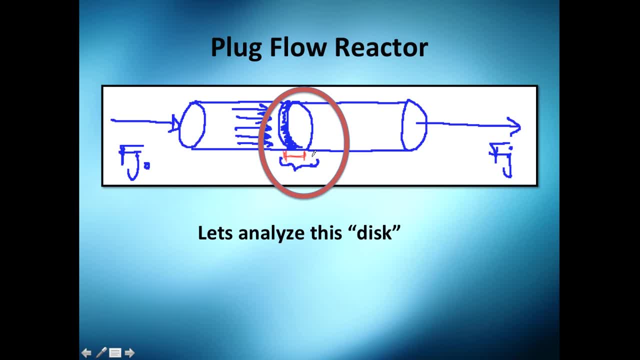 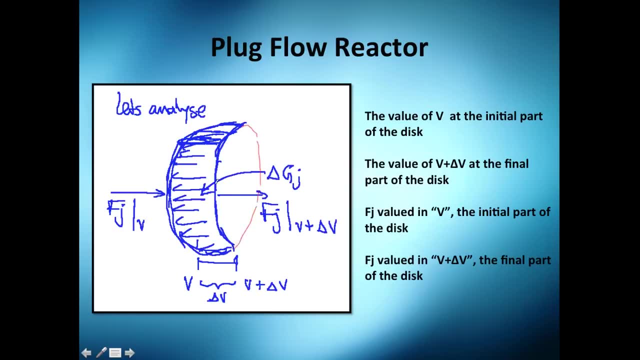 I've learned from mathematics is that everything is beautiful in the differential world. So yeah, we got this disk. let me explain you a little bit. so this is the tube here. we got this diameter. you don't need it, but of course this diameter. you got this inlet. 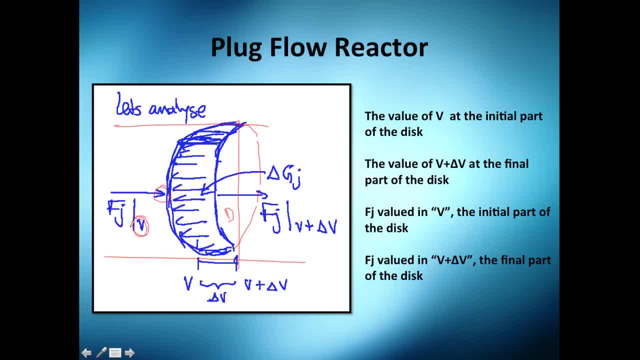 which is the flow of jet. The flow of jet evaluated in this volume here and the flow of jet evaluated in this volume plus the change in volume. Where is the change of volume? Of course this little disk has a change of volume, so we have one volume here. and if 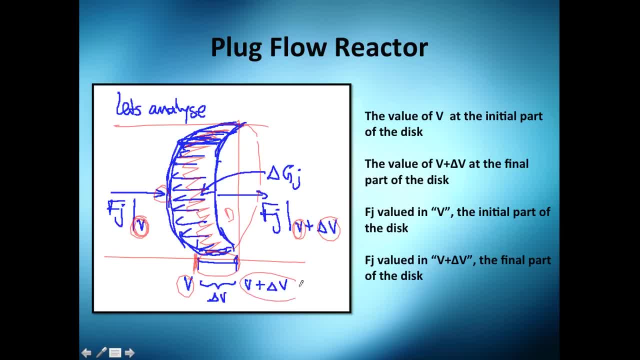 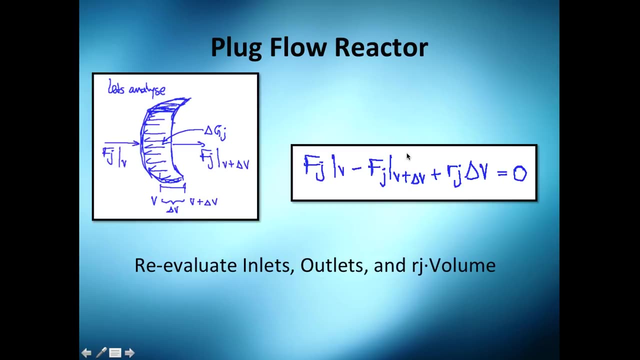 we add this little volume here, we will have volume plus the change of volume, And this differential disk has also a change or generation concept. So read this part, This part, slowly, because it's a very conceptual part, but we are going to be able to form. 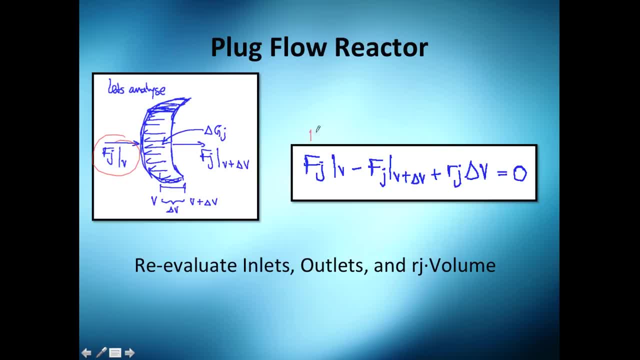 a new concept. So the inlet, this is the inlet, My flow of jet evaluated at this certain point. Now the flow of jet at the outlet will be this: one volume plus the change in volume, Now RRG, which is the generation. 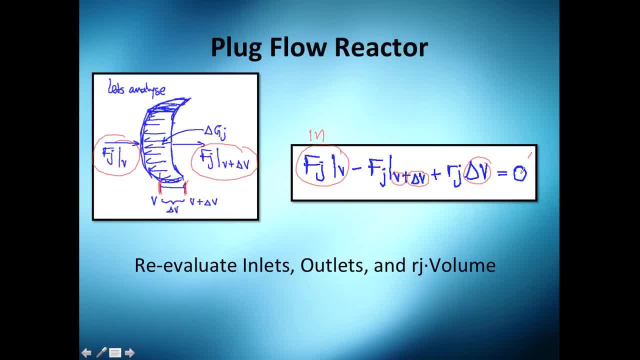 This generation is simply times the change in volume And because it's accumulation, we have no, since it's continuous, we have no accumulation concepts. So let's re-evaluate inlet outlets and the generation concept and we get this thing right here. 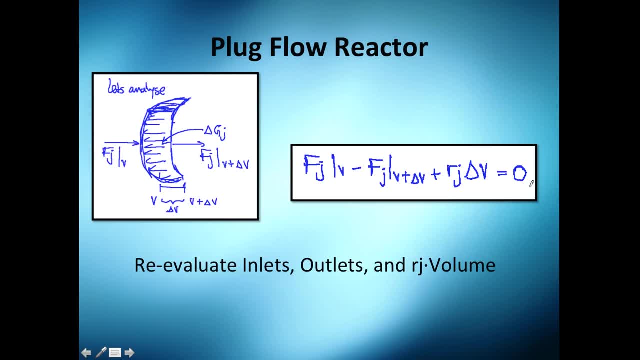 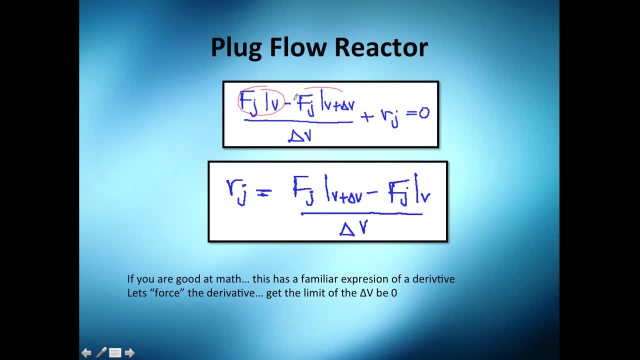 Well, sorry, this one, And what I'm going to do is essentially divide everything by the change in volume. So this inlet and this outlet are divided by the change in volume. I use this one. This is the change in volume. I used to have a change in volume here, but since I divide it by the change in volume, 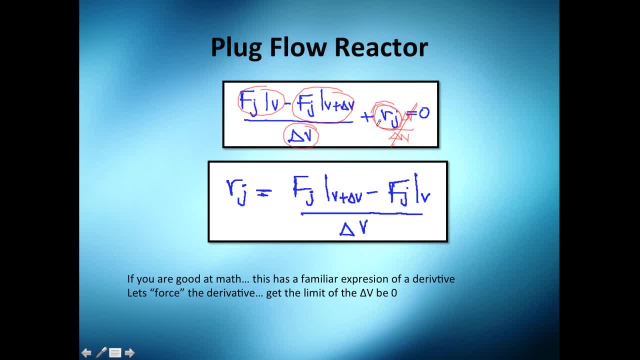 I take it away. And I'm going to take away this value, the rate of reaction. I get it here, And if you are good at math, or at least you remember this form, this has a familiar expression of a derivative. So let's force that derivative. 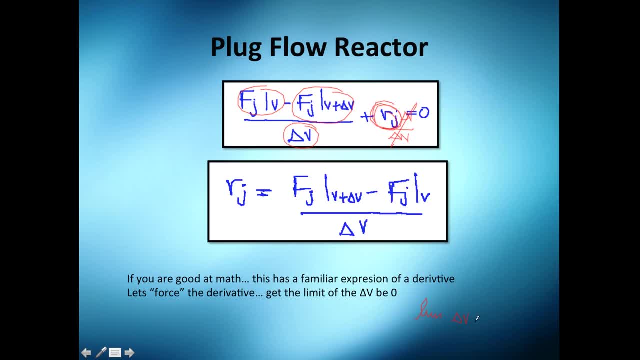 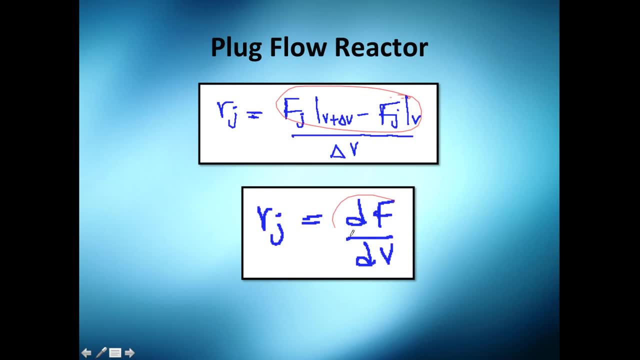 What do we need to do with the limit, as the change in volume goes to zero? That's the definition of a derivative. So this here will be a difference. Okay, This here will be a differential of flow and this here will be a differential of volume. 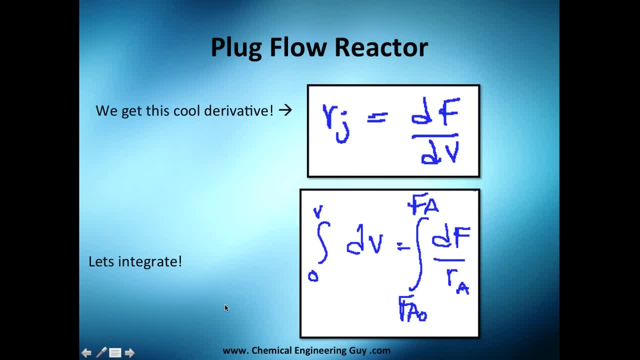 That's the rate of reaction. And yes, guys, we are done. This is our design equation. If you want to integrate it, you can do it. You just need to change this one here, And since this is dependent on flow, you can change it. 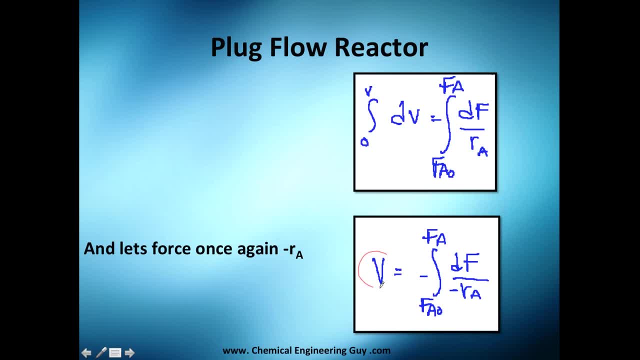 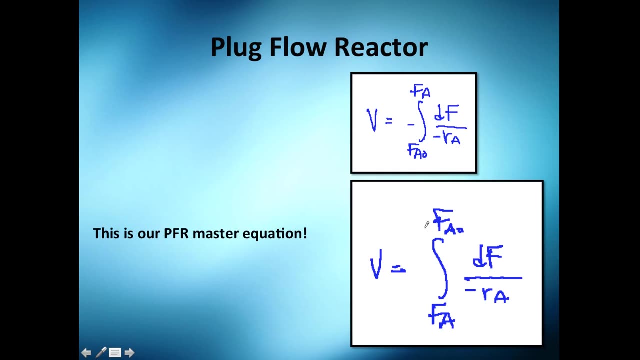 And you will get something like this: In terms of volume, you get an integral. And remember we love this is positive RA, but we want negative RA or rate of reaction here, So we force it. So that's my actual equation, this one here. 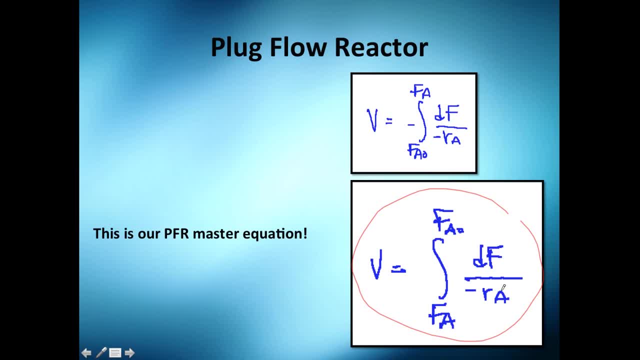 I like it because you got volume, you got the differential of flow, so that actually depends on how the rate of reaction law is. It can be as simple as one constant, so it will be easy, but it can be as complicated, as I don't know the flow of A to the square time, to concentration. 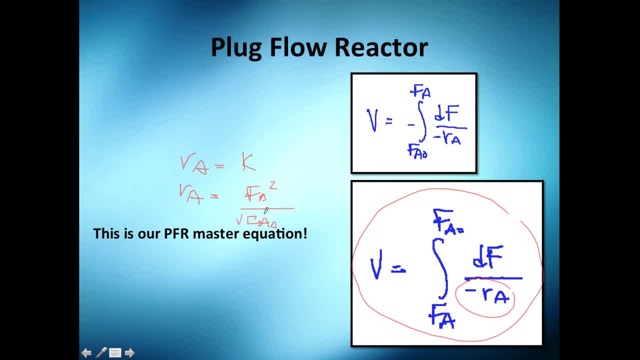 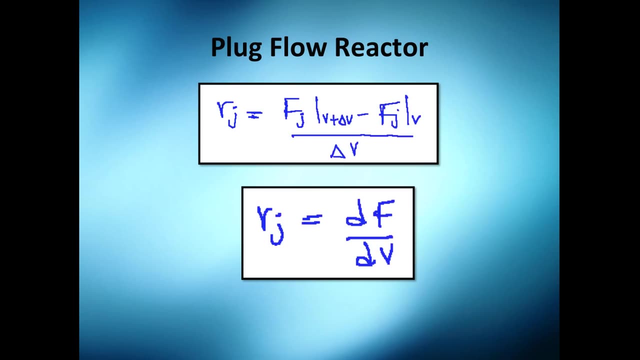 The concentration of that number here to the square root. and yes, this will be kind of complicated to do, but you can do it with numerical methods. And yes, we're done with the PFR. That's the master equation. It's a little bit more complex because you need to know more about this little disk.